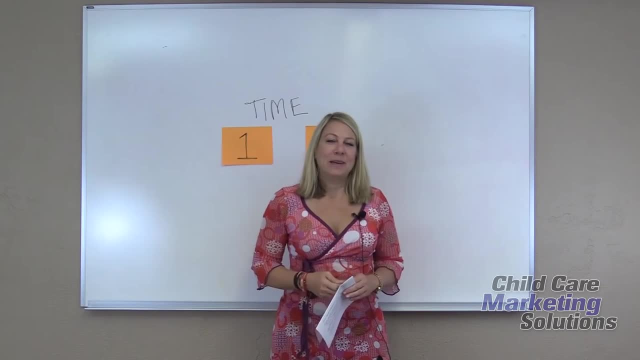 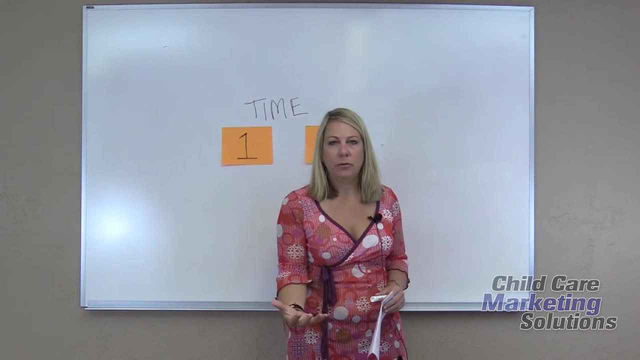 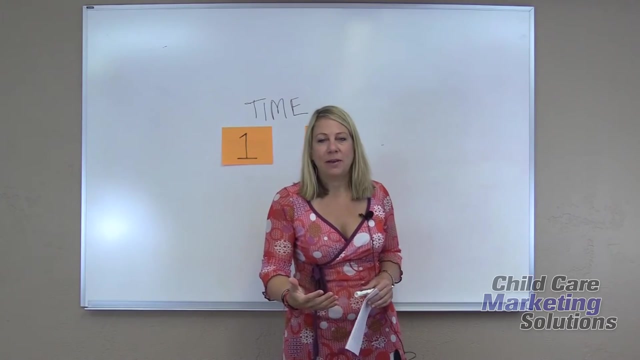 coached one of our Platinum Plus members, Matt from Indianapolis, on how to get a handle on his time, because he was just again, like many of you, completely just walking into his schools and getting interrupted, Interrupted, pulled, fighting fires and not focusing on his high payoff activities And 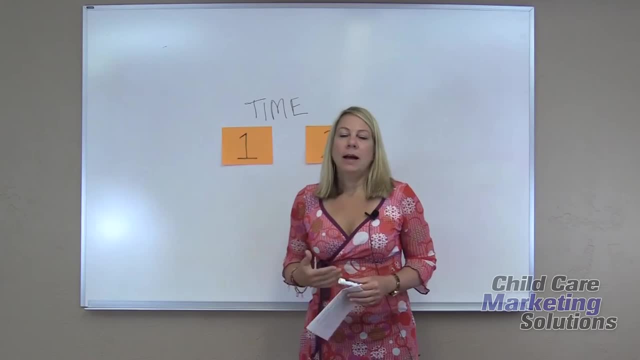 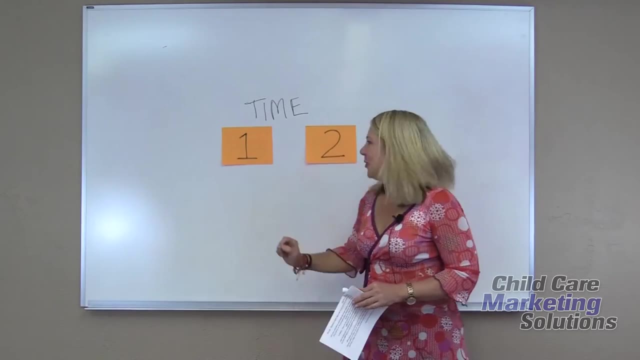 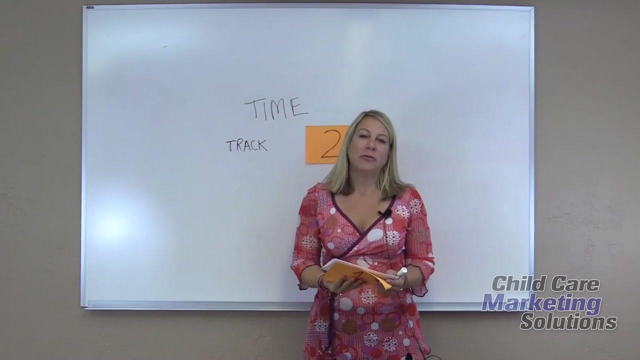 we talk about that a lot here in the Child Care Success Academy. So I counseled Matt to actually do strategy number one here behind the magic orange curtain, and I'll reveal that, which is simply to track his time, And big kudos to Matt for actually doing it. And here: 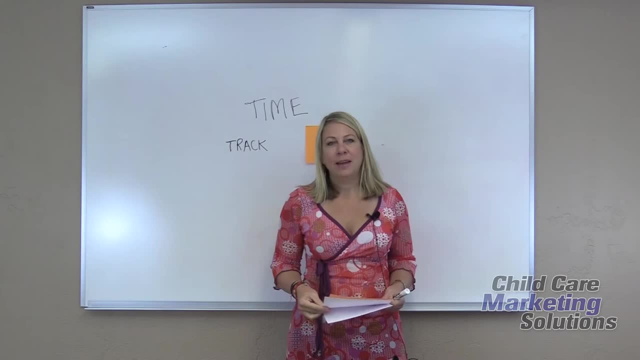 in this video, we're going to share with you a quick screenshot of his initiative, And I'm going to show you a screenshot of Matt's initial tracking spreadsheet that he created, And so what I want you guys to do to get a handle on your time and figure out exactly. 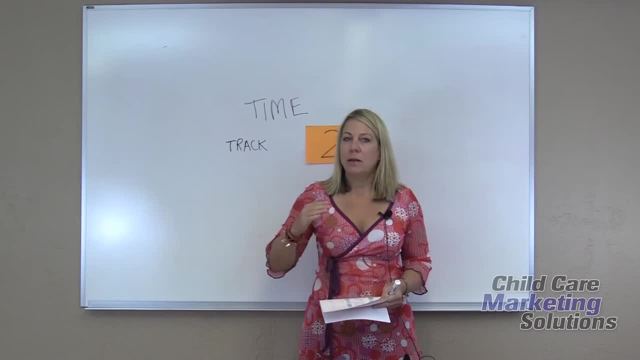 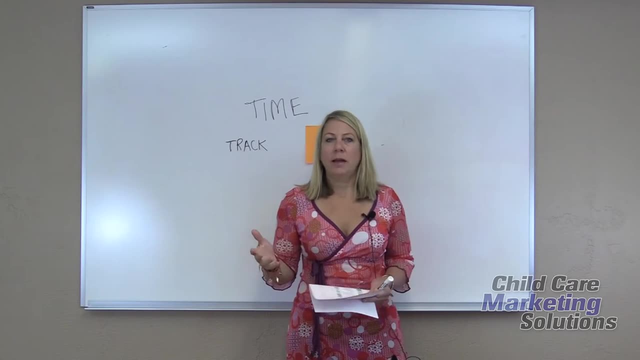 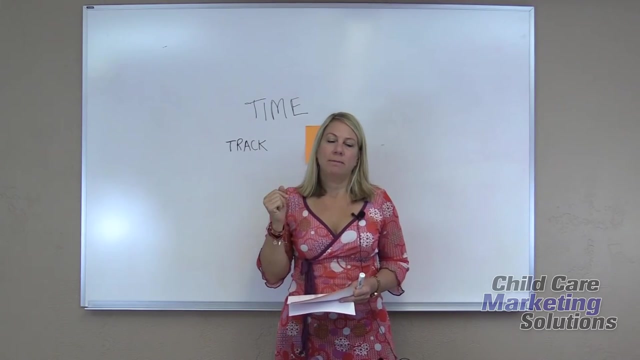 how much time you're really spending on the stuff that's going to move your business forward, versus emergencies, interruptions and other issues that aren't going to move your business forward. necessarily is to track your time So you can see that Matt's tracking spreadsheet. 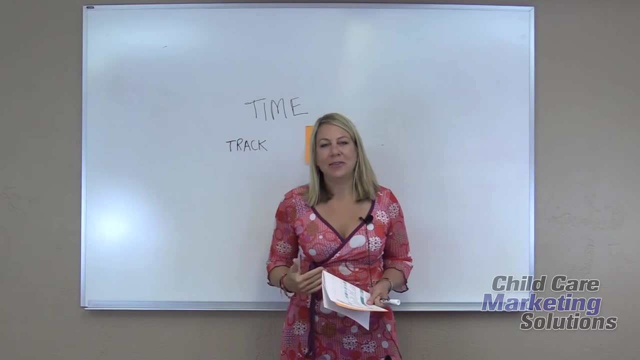 he started out just in a simple way, And what I recommend is just to write down your exactly what you've done every day on a yellow pad of paper on your desk. just track it. You can do it electronically if you want, but you could just write down how you spend. 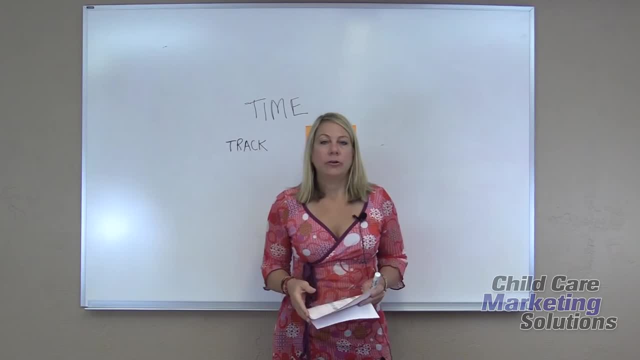 a week. just start with a day and a week in your life, And Matt actually did it for a full month, So he tracked 180 hours of activity over a four, four and a half month long period. four and a half week period. 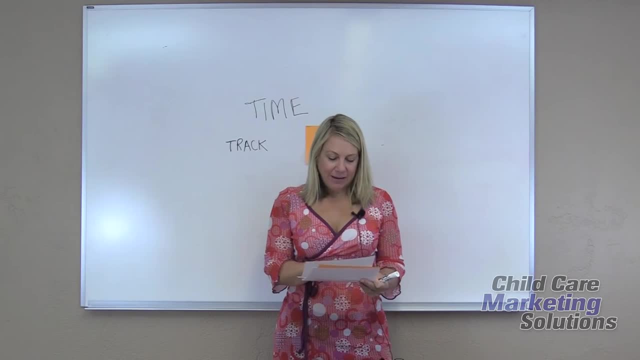 And so, of his 180 hours, he realized that 18% of his time, or 32 of the 180 hours, was spent on a given emergency that he had to deal with that month. Now is every month going to be like that, Probably. 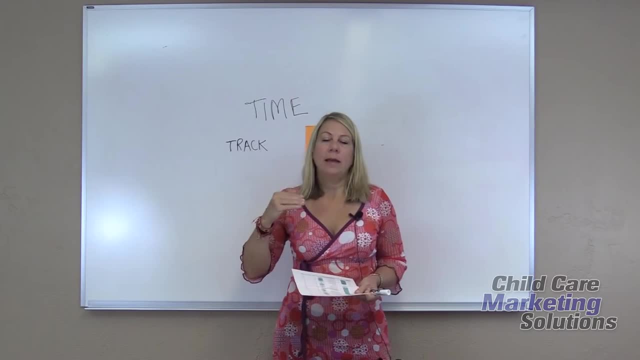 not, but now he's got more insights and awareness to when he's spending unneeded time on emergencies. And so from there we talked about: well, how can you train your staff and delegate those emergencies A you don't have to micromanage them, because you can empower your staff to handle them. 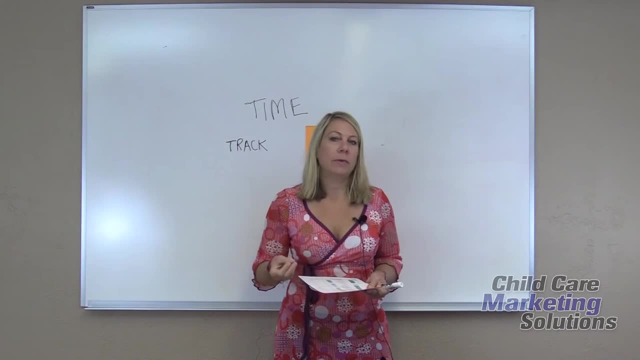 And B, make sure that they're well-trained and that you have policies and procedures and operations manual that supports you through those emergency situations. 90,, 95% of the time. So that was an insight which is geez. I spent 18% of my time on emergencies, which 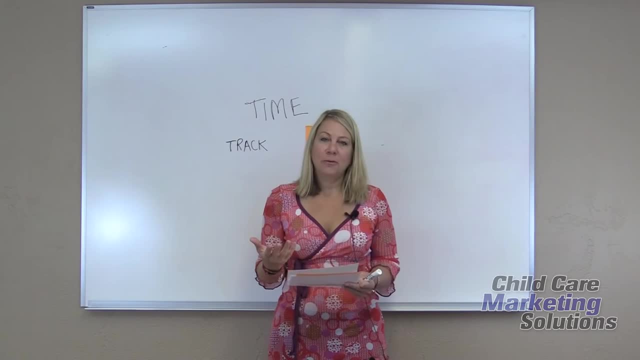 was not good. He only spent 6% of his time on his big goals and 2% of his time on the training that we provide and trying to market his schools. So that was pretty rough, because only 8% of his time was really spent on trying to move. 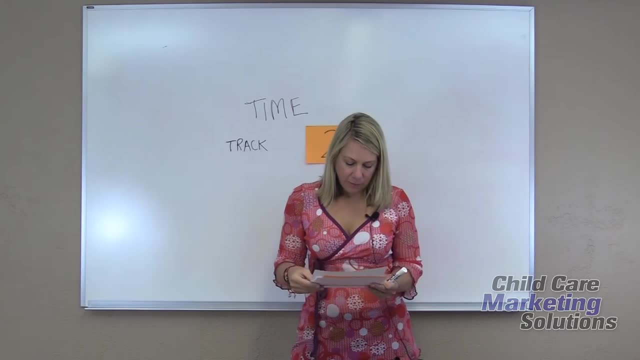 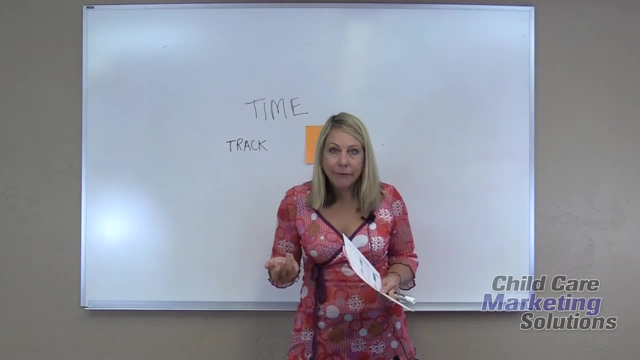 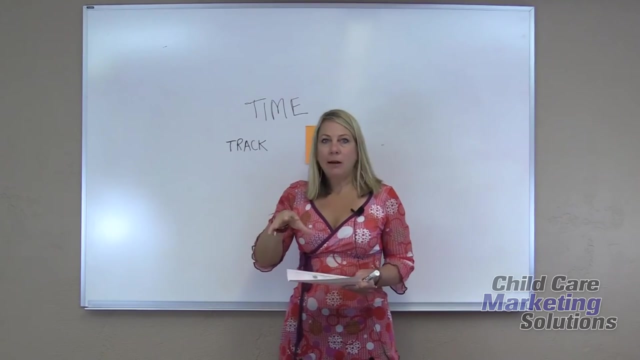 the business forward and 18% on emergency And a bunch of other time spent on billing and HR and general stuff that isn't moving his business forward. So tracking your time and just doing a simple pad of paper exercise if you want to transfer it to a spreadsheet. 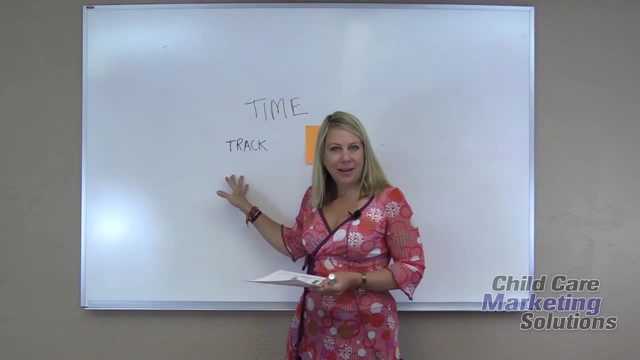 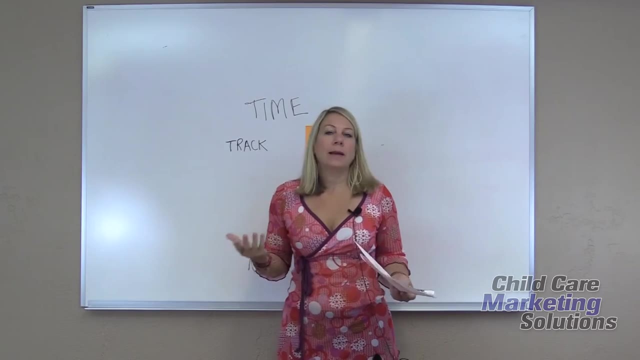 great. So that is going to give you a huge amount of clarity in how you're spending your time and how you're getting interrupted, And then you can frame it to now: what am I going to do about this, right? But first you've got to know, You've got to have the clarity on 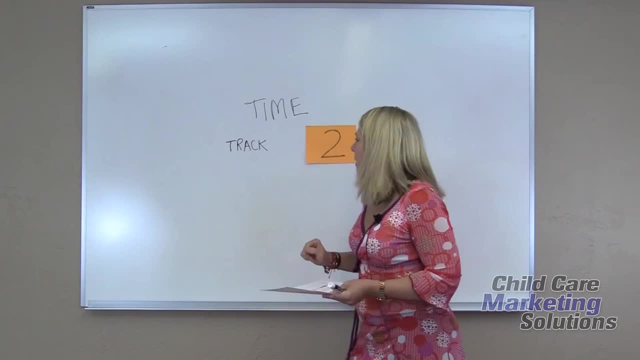 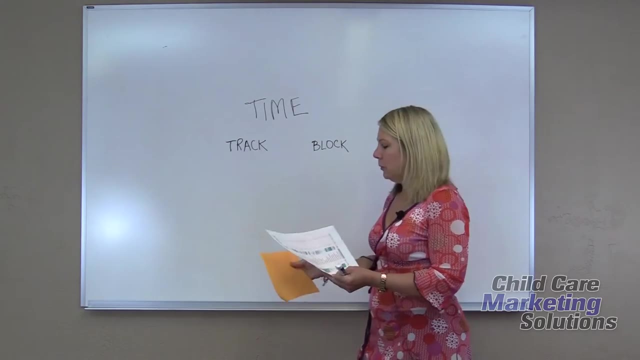 really what you're spending your time on. So that's the first secret. The second secret is: well, let's reveal it, shall we? It's to block, So we teach time blocking Everybody on our team here at Child Care Marketing and most of our clients they. 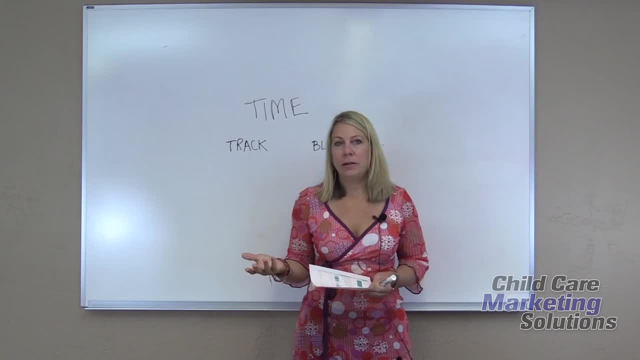 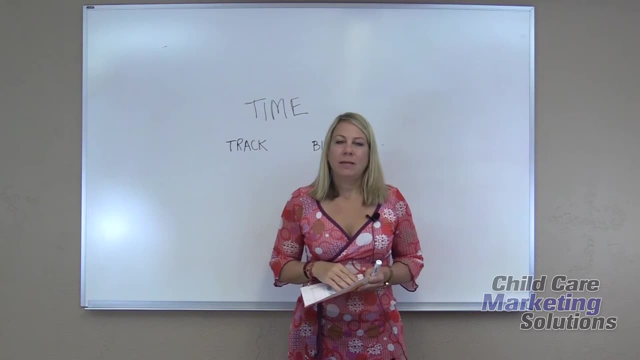 use time blocking And it's really as simple as you have to have an electronic calendar really to do it effectively. You can time block using paper systems, but it's more difficult because with time blocking, basically you just look at your priority list, You look. 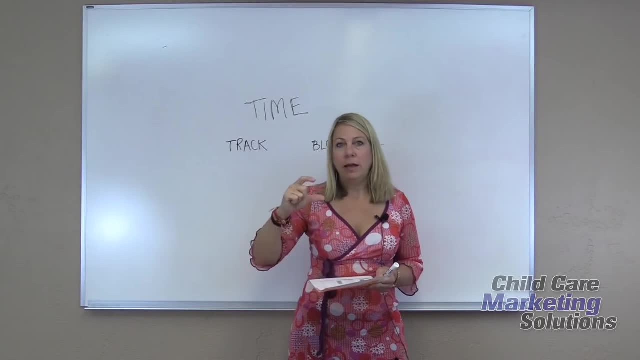 at what's going to move your business forward right. And then you take those tasks and those steps and you say this is likely going to take an hour, so I'm going to block it into my calendar. And then you're vigilant with yourself about to those blocks You can. 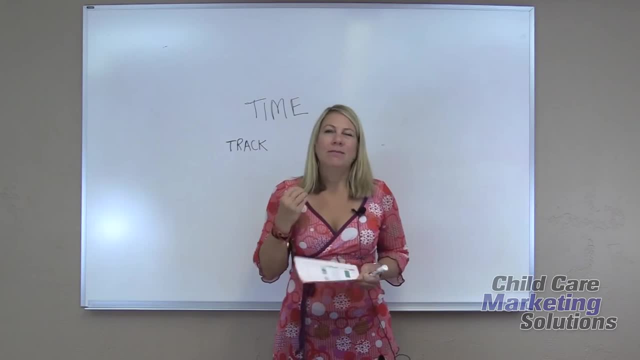 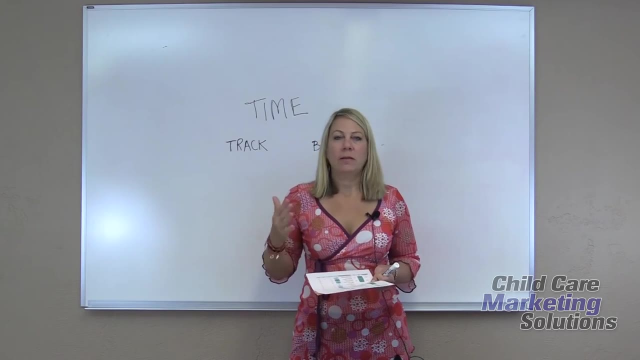 move stuff around. I move stuff around, for sure, but I would say 80% of the time I'm vigilant to sticking to those blocks when I block them, so that I can make sure I'm hitting the stuff on my to-do list that's going to move the business forward. 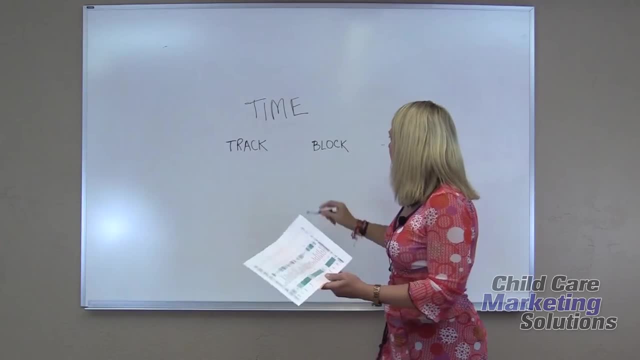 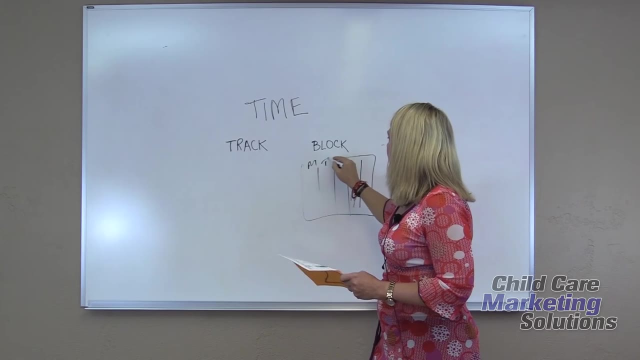 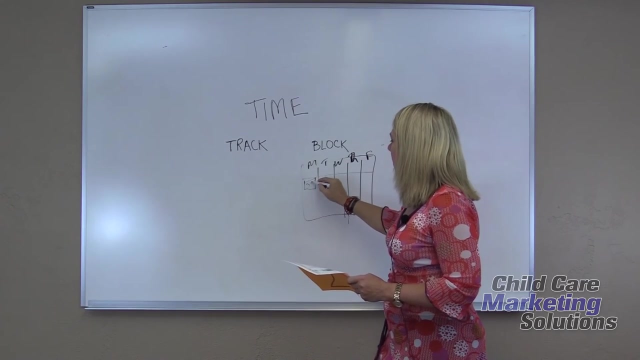 So using time blocking, and it really just looks like you've got a Monday through Friday, let's say Google Calendar or Outlook, and you've got your day here and you just go in. Oops, Thursday You just go in and you block it in. So you're like 9 to 11, and you're 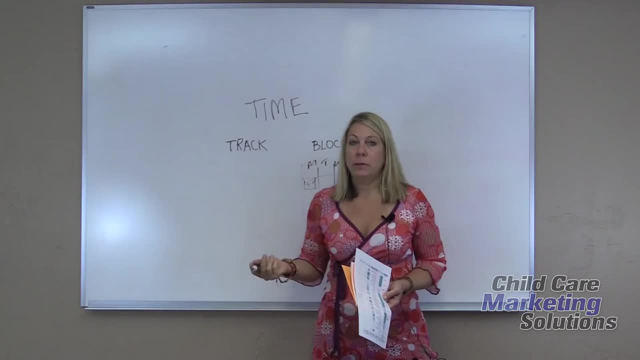 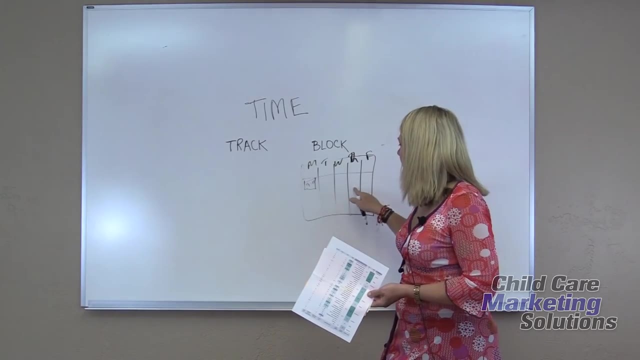 like I'm working on my marketing plan or my calendar or enrollment building efforts for the fall, or my summer camp for next year or whatever. You can put your team meetings in here, your one-on-ones in here, and it's highly effective. And so if you're not using 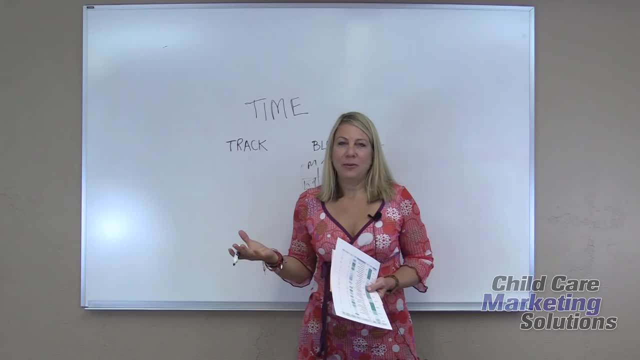 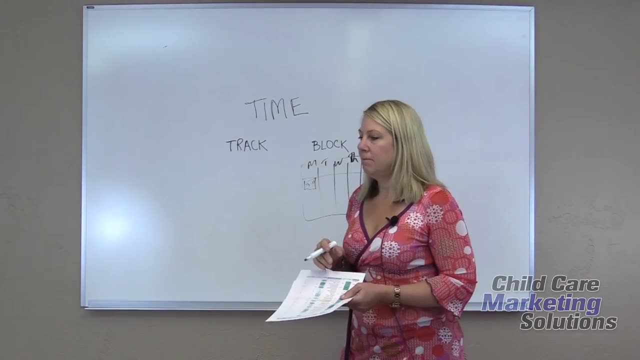 time blocking. it's probably the most effective strategy that we teach of all of the – and we have nine or ten strategies that we teach for how to get out of overwhelm and how to make your time more effective. Again, we all have 24 hours in a day. 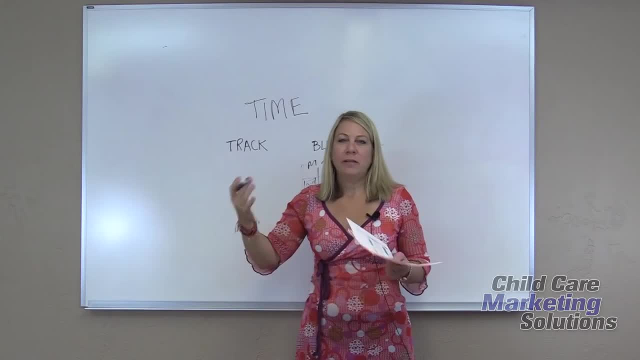 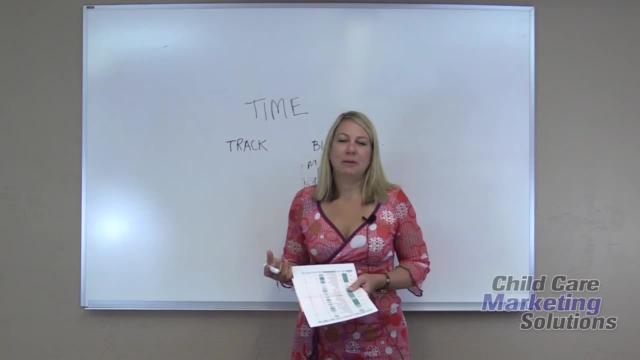 So how can people like Richard Branson and other hugely successful and high-performing entrepreneurs get so much done and yet still have time to enjoy life in Necker Island and live a full life? And this is the key guys. This is the key to living a full, balanced. 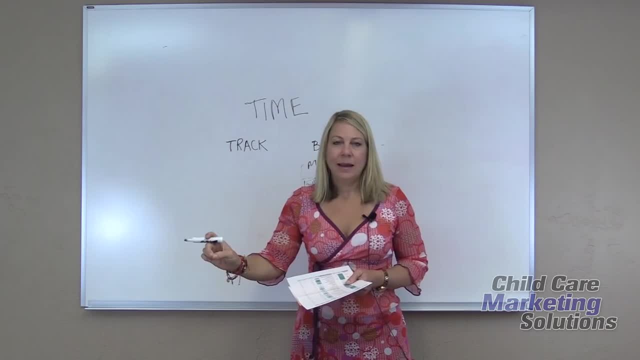 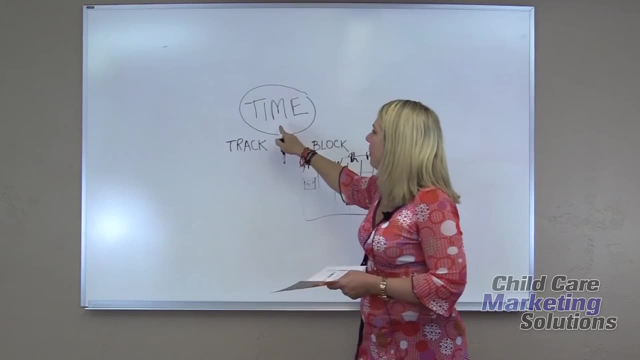 life with your loved ones and your business, not driving you crazy and not making you work 60 hours a week. So just get started with these two ideas and you will start having clarity, Which is the key to success. The first thing you got to do is have clarity on how you're. 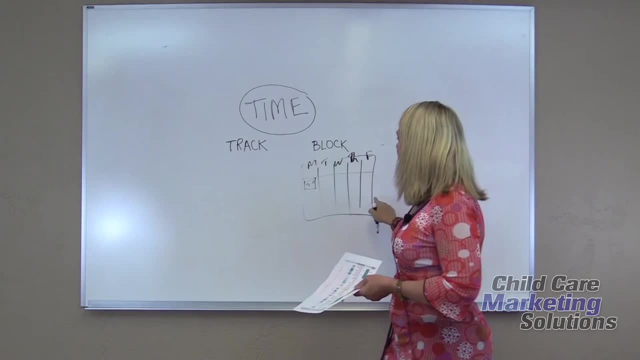 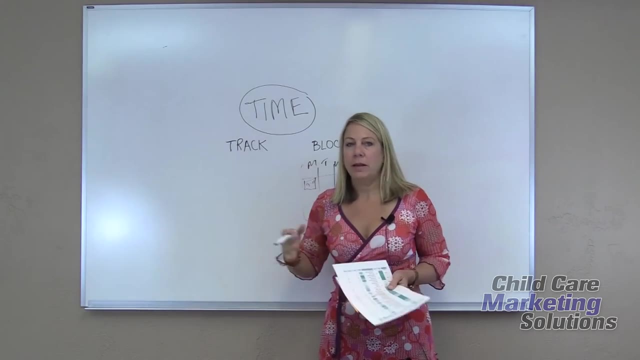 spending your time and then blocking your time and then sharing this with your team, Sharing your calendar with your team using Google Calendars. That's what we do, So everybody on our team has a calendar and we can all see where each other are planning to be when. 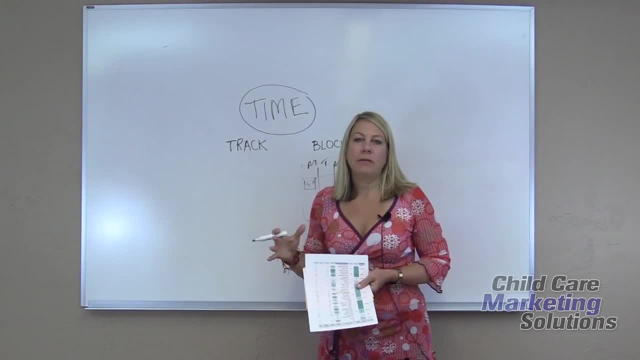 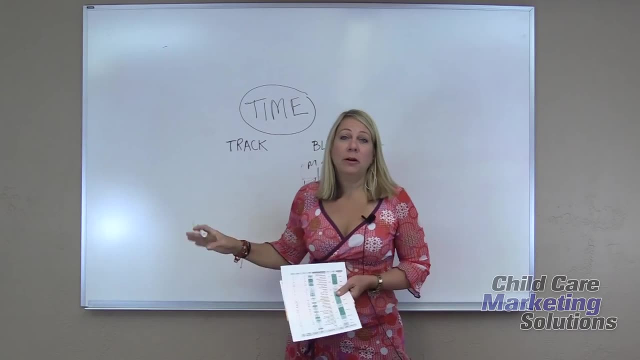 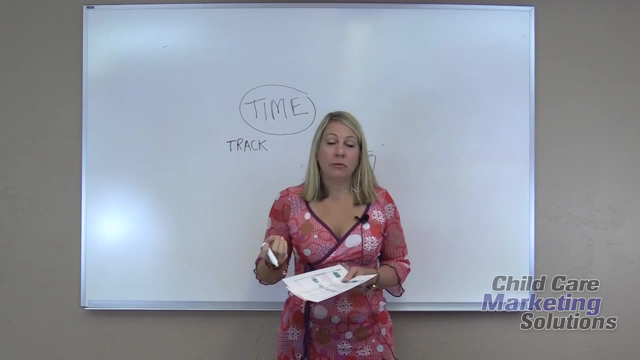 they have meetings, when they have calls and what they're working on, So it's a highly effective management tool as well. So these are two strategies. We teach seven or eight more. Now we have a newly revised course, a training system for you, called The Ultimate Time Management. 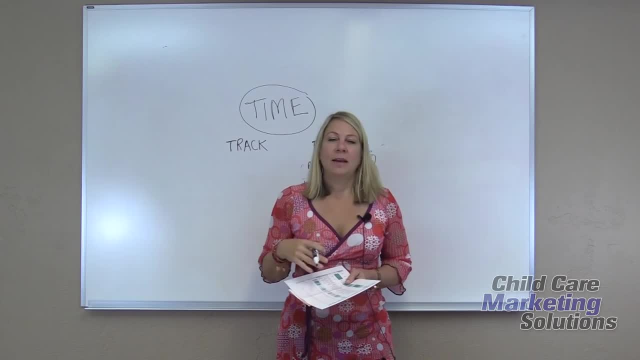 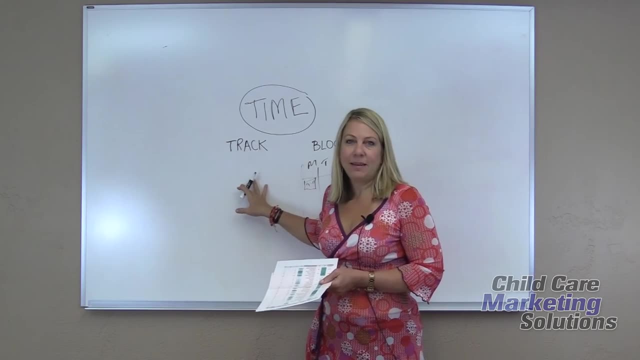 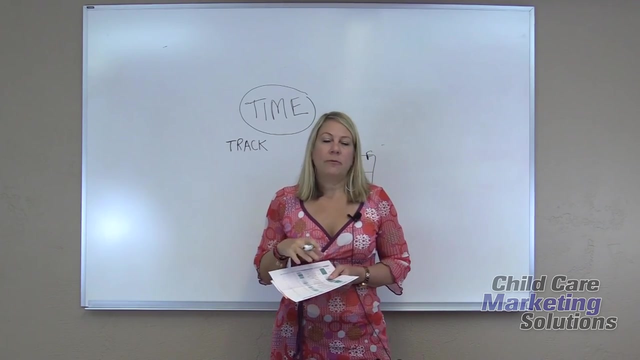 Guide for Child Care Leaders and we just updated it. Jessica and I reveal the other seven or eight strategies around time management. So if you want, if you like this and you want the other strategies and help, you can go to child care dash marketing dot com forward.